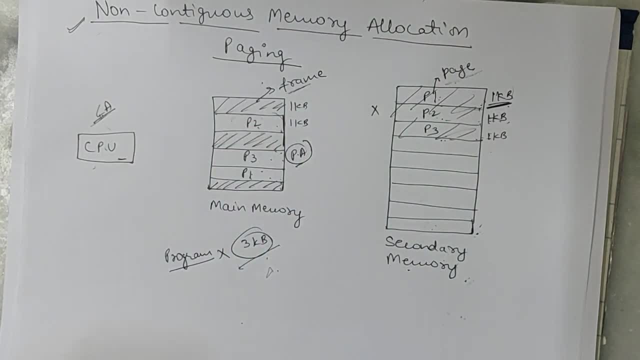 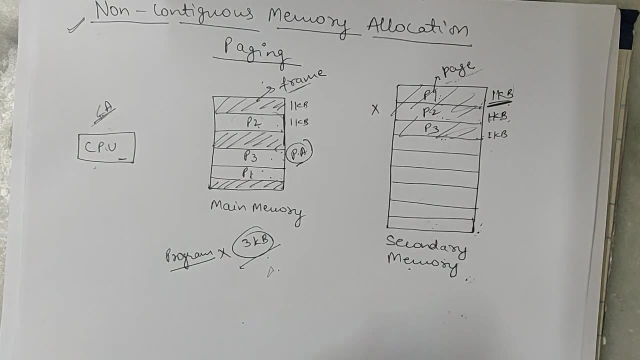 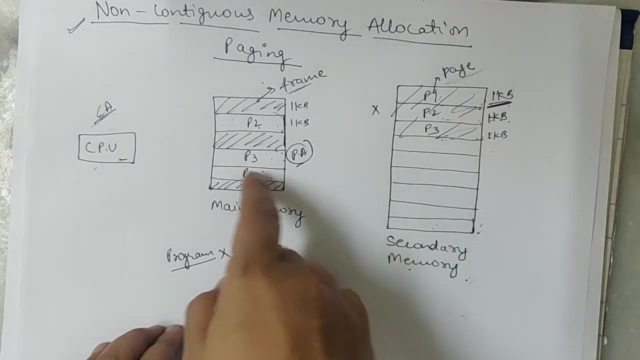 it in the secondary memory and from secondary memory it will load it in main memory. Suppose we have a program x which is of size 3kb. we cut that program into 1kb size 3 pieces. each piece is of 1kb and here the size of partitions is also 1kb, Similarly the size. 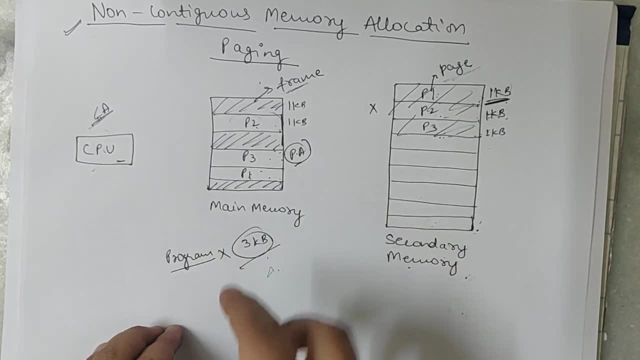 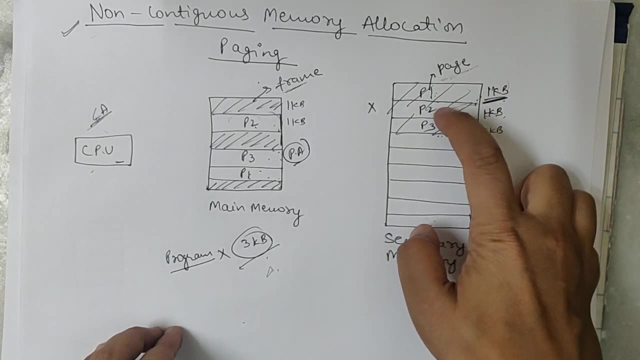 of main memory partitions is also 1kb. So we have made 3 pieces of our program of 1kb because our program size is 3kb, so we have made 3 pages of it. Page number 1 is loaded here, page number 2, page number 3 and each partition is of size 1kb And every second. 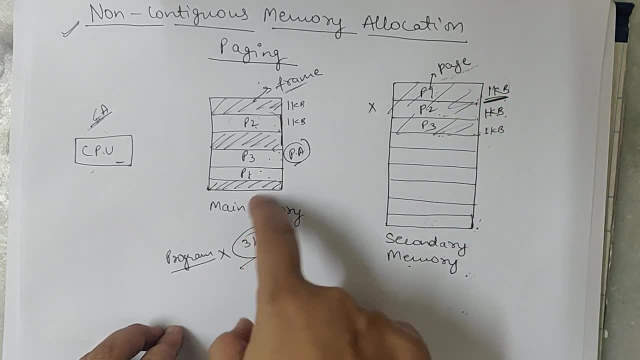 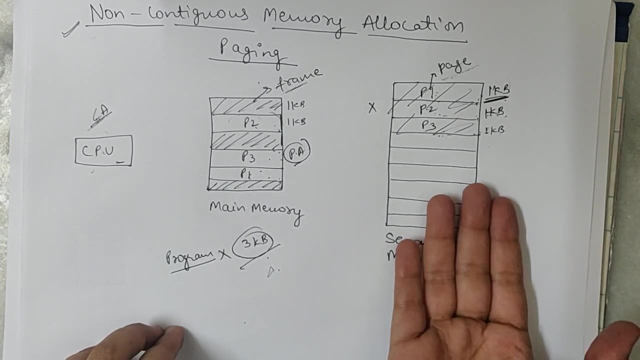 memory partition is called as page and every partition of main memory is called as frame. Here also 1kb size is there, and here also 1kb size is there. So what we are doing in paging Program x has to be executed. and how many pages are there in program x? Page 1, page. 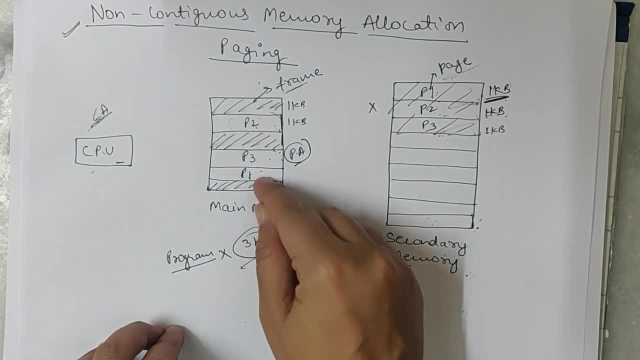 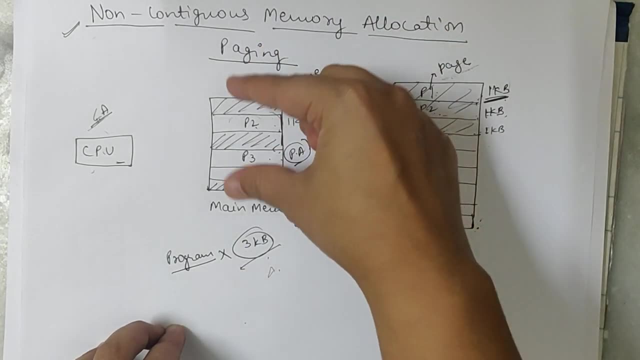 2, page 3.. So, as it is, these pages are loaded here: Page 1,, page 2,, page 3.. Now CPU will pick and execute the pages one by one, So our entire program is being loaded from secondary. 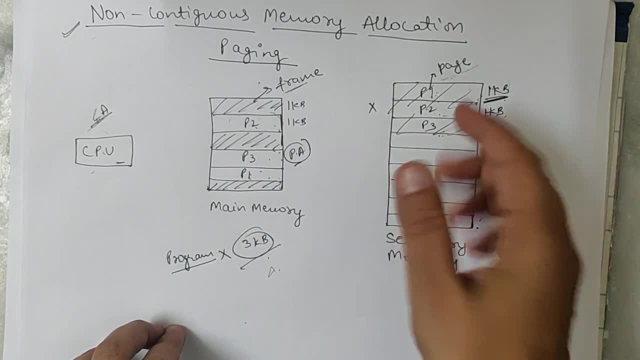 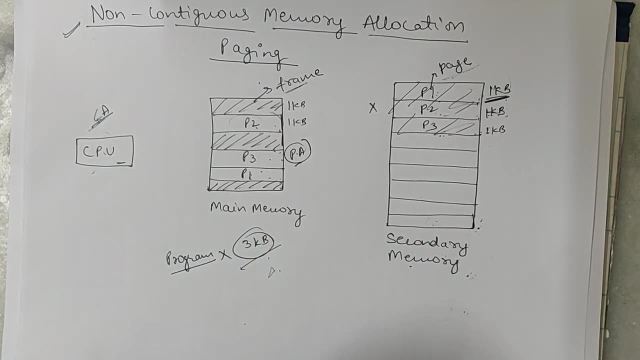 memory to main memory, Because program x is of size 3kb So we have to load all the pages. So in program x there are 3 pages, So all the pages are being loaded in main memory. So what is demand paging? We are getting to know from the name itself that when the page 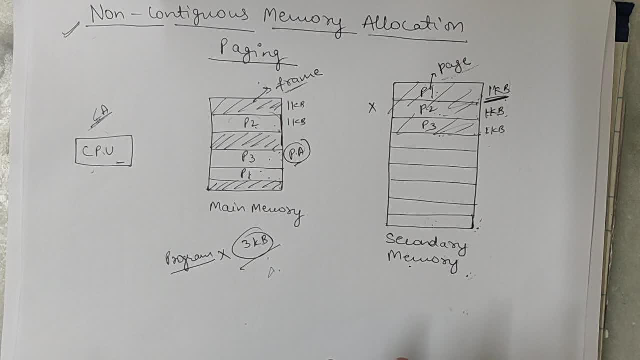 is in demand, then load that only. There is no need to load all the pages: Page number 1,, 2,, 3.. So there is no need to load all the pages. This is just an example. It is possible that there are 20 pages in our program, So 20 pages of 20 pages will not be executed. 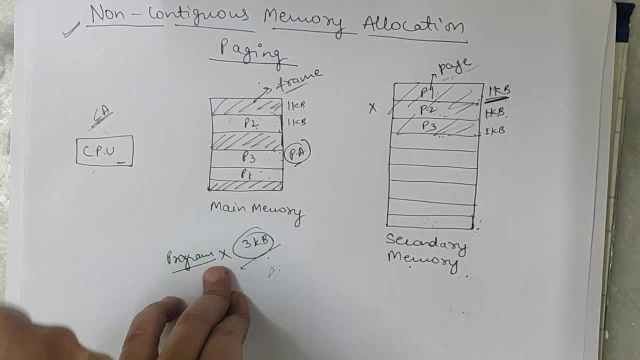 together by CPU. It will be done one by one Because pages are loaded in main memory, So there will be particular instructions in it. Every page has 10 instructions. So if there are 10 instructions in page 1, then it will execute the first instruction, then second. 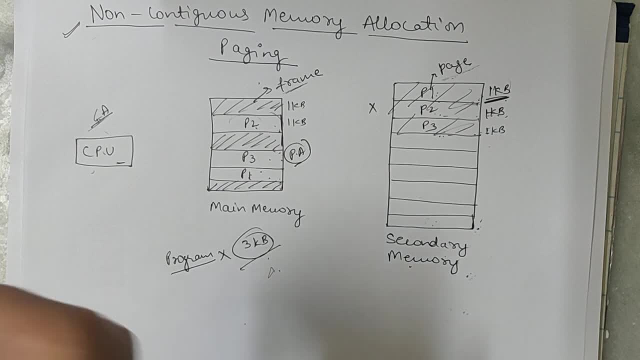 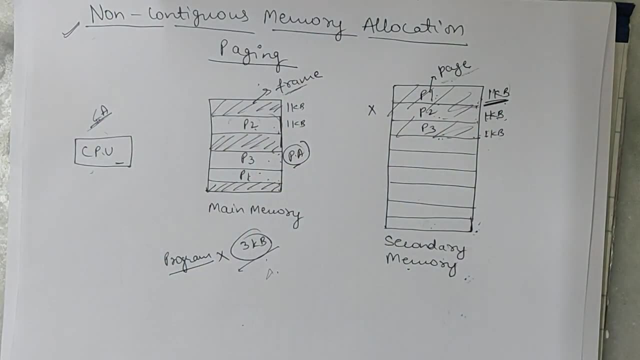 then third. So if there are 20 pages in any program, then what is happening in paging In secondary memory? there are 20 pages. So, as it is, 20 pages are loaded in main memory. CPU is then executing it. But what is demand paging, saying Work on demand. The page on. 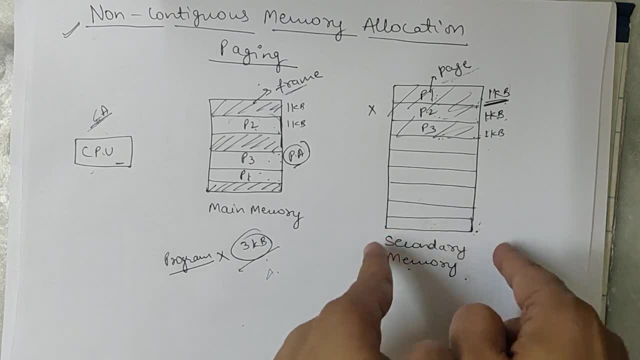 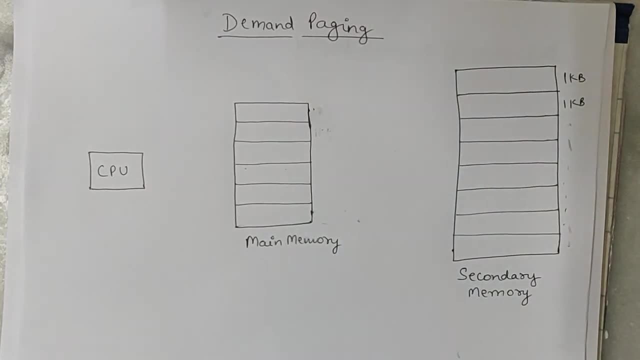 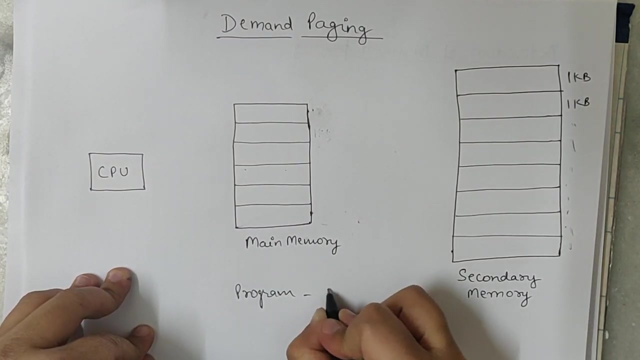 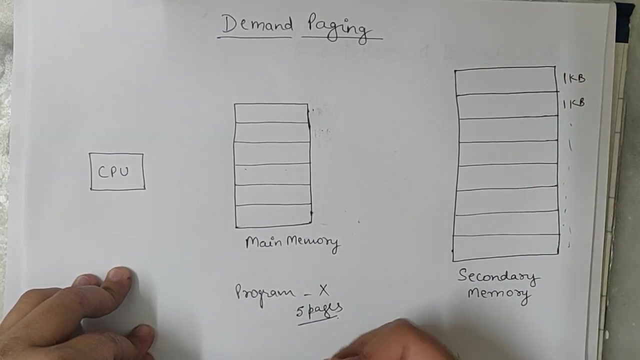 which CPU has demand, that same page will be loaded from secondary memory to main memory. There is no need to load all the pages Now. we will see it with a diagram. Our program is, its name is x and it has 5 pages. All these are of 11kb, So it will be of 5kb size. 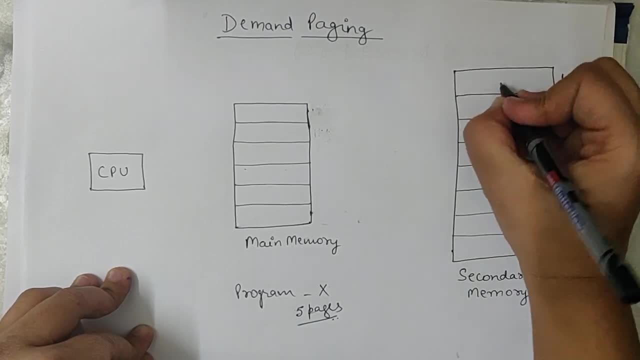 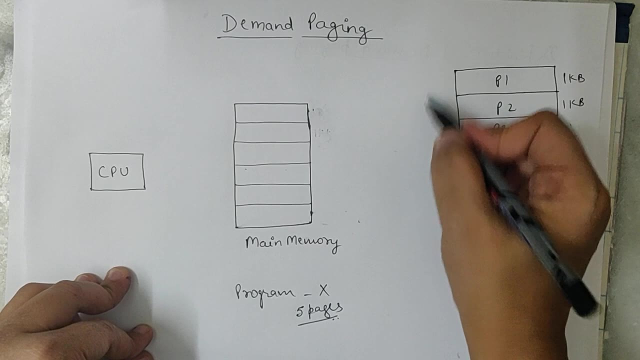 We have made 5 pages of it. We have put p1 here, p2 here, p3 here, p4 here, p5 here. The program x has taken its place, Okay, And here also there are many sizes of 1kb in. 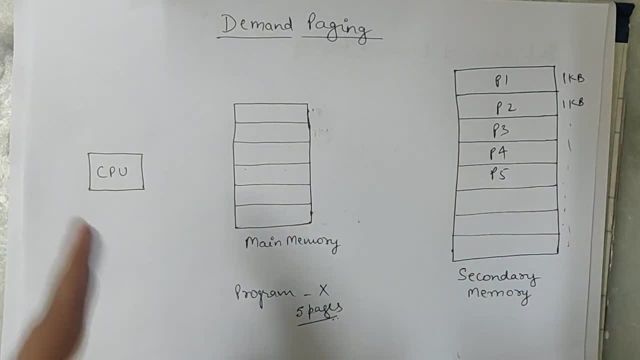 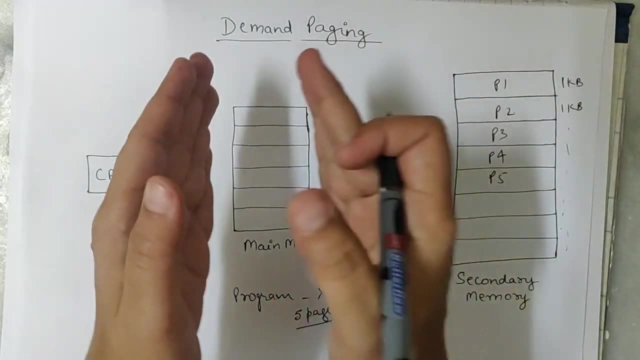 main memory. What was happening in paging As soon as CPU had to execute program number x, then 5 pages of 5 were loading here in secondary memory: Some page 1 here, 2 here, 3 here, 4 here, 5 here, Because everyone's size is 1kb. Here also there is 1kb There. 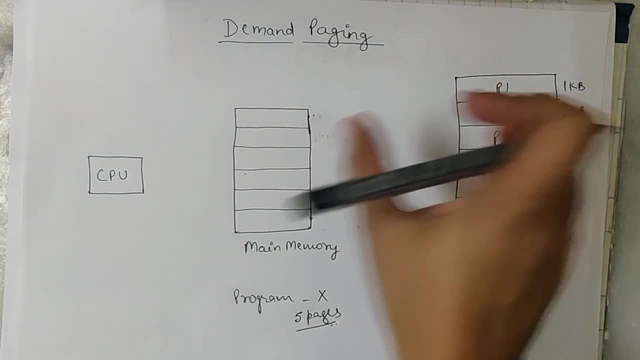 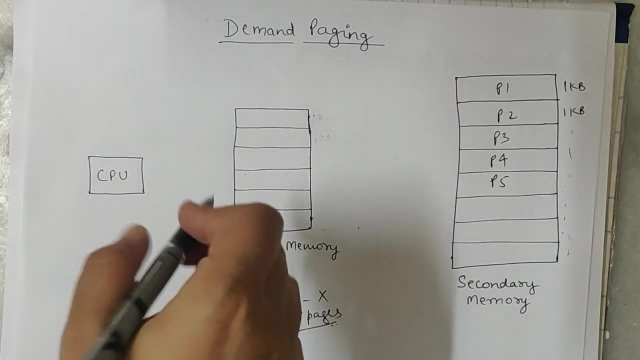 will not be external or internal fragmentation, Because the size of every partition is the same. So these pages. now what was happening in paging? All the applications were loaded as it is and then CPU used to pick the page from here and used to execute the particular. 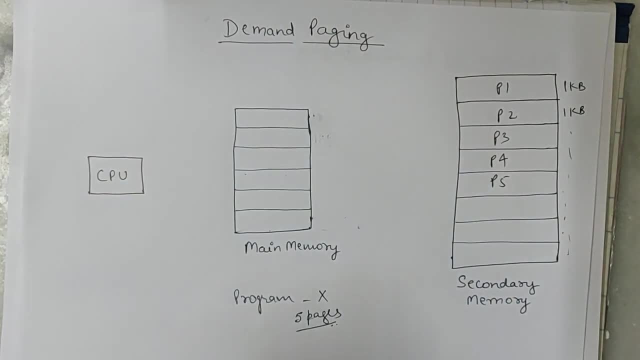 instruction, But demand paging, which is demand paging. it says don't load all the pages At the same time. load the particular page in the main memory, from the secondary memory to the main memory of the particular page. What will happen with this? Space will be made. 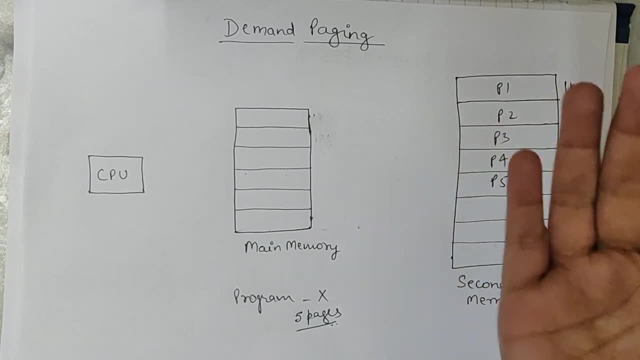 in the main memory. Okay, If you have 20 pages in any program and if you load all 20 pages in this, then the chances of the main memory being full will be high. So if you load 20 pages in this, then the chances of the main memory being full will be high. So if you 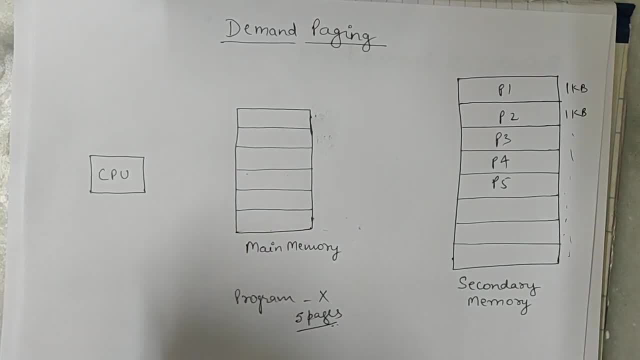 load 20 pages in this, then the chances of the main memory being full will be high. So if the pages get 특ited then you want to use the main memory efficiently. then the demand paging is the concept will be look like demand paging if you want to use the main memory. 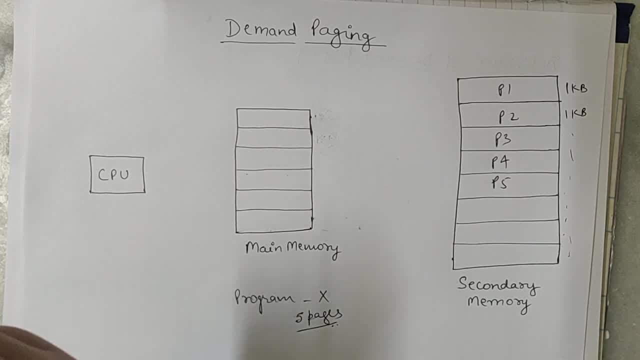 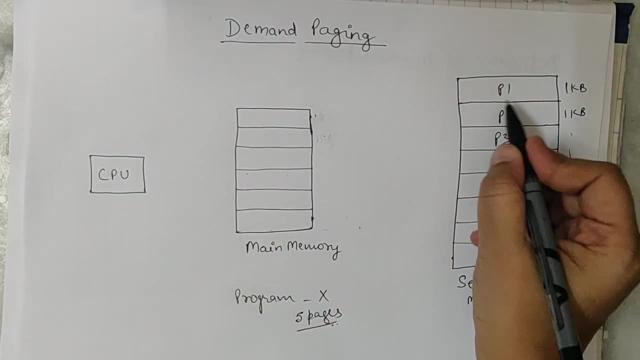 effectively, then when the domain is in demand, that page should be brought in the main memory from the secondary Up to. if CPU says that I want to execute page no.2, then you should bring page no.2 only from the secondary, from the main memory. Don't load all the pages. 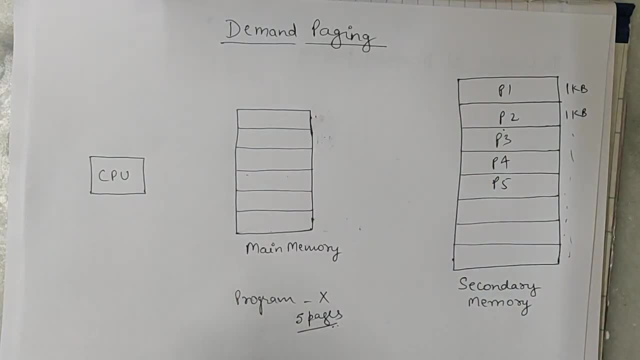 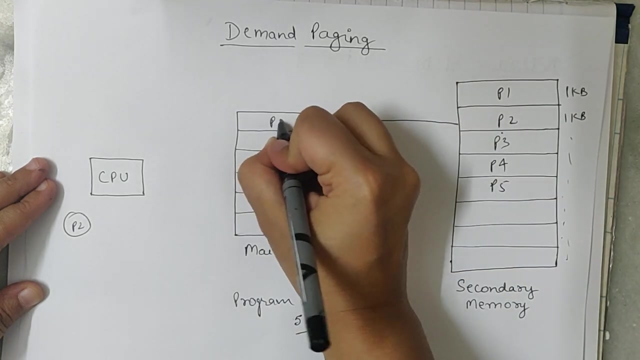 in one place. so this is the only difference between pages being sufficiently used Here, difference between paging and demand paging. So what happens in demand paging? Initially our main memory is empty. CPU said: I have to execute page number 2.. So page number 2 is in main memory. 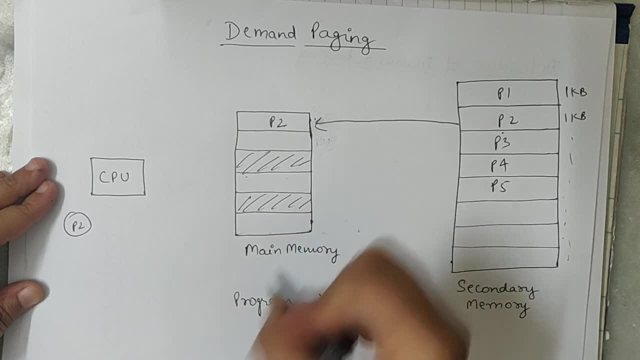 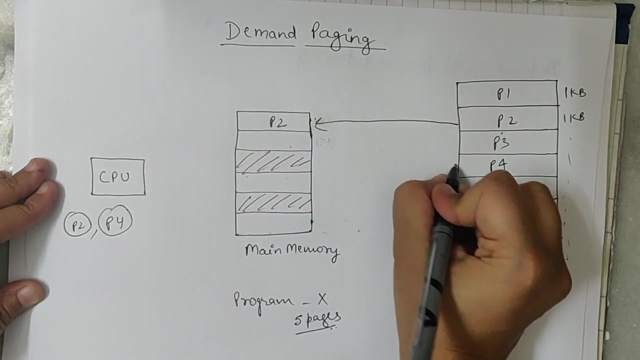 Suppose, in main memory this space is occupied and this space is occupied, So we put it here. Now CPU will execute instructions from page number 2 and will give us output. Now CPU said I have to execute page number 4.. Where is space empty? So page number 4 is here. 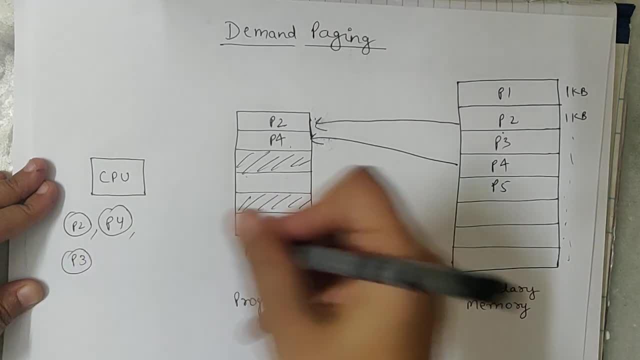 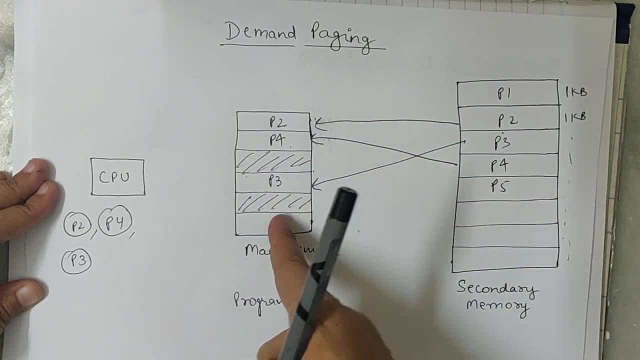 Now CPU said I have to execute page number 3.. Here space is not empty, So page number 3 is here. If I have to send any page back to back-end in secondary memory, then we can do that also When any page comes here. 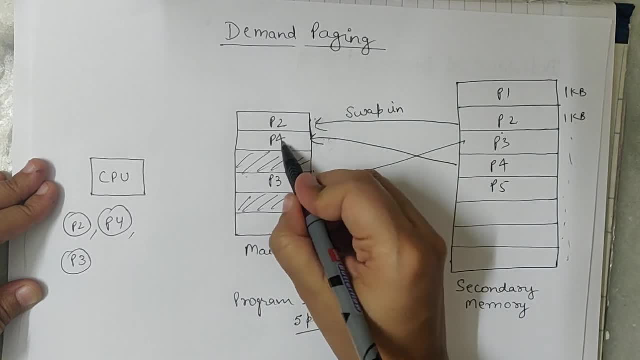 we call it swap-in. Now suppose I have to send page number 4 back here, So we can do that also. When any page comes here, we call it swap-in. Now suppose I have to send page number 4 back here, So we can do that also. When any page comes here, we call it swap-in. Now suppose I have to send page number 4 back here. 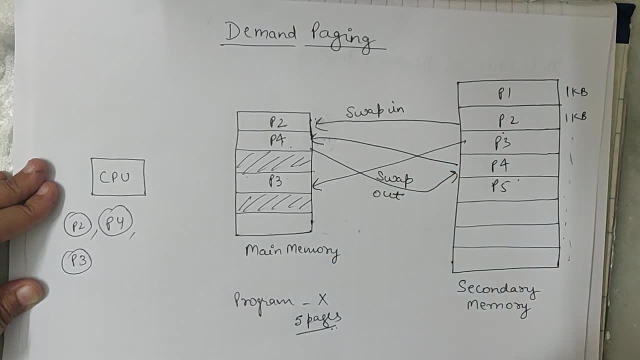 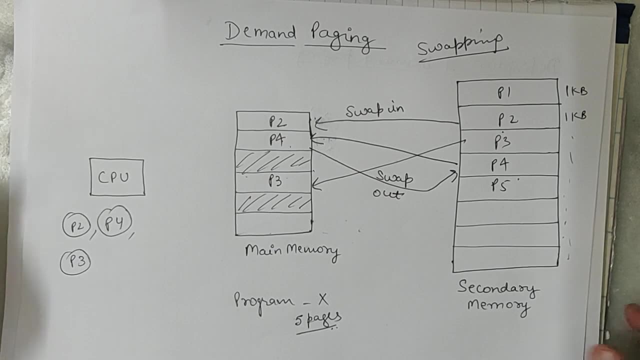 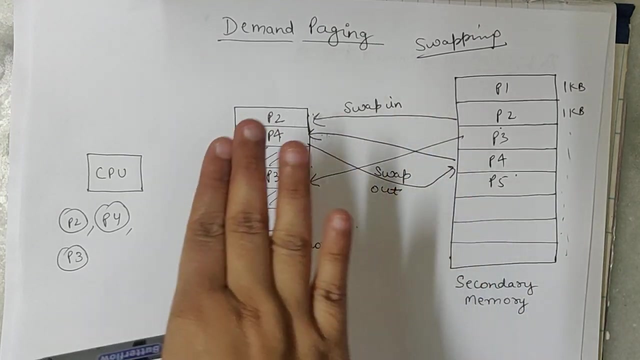 If this happens, then we call it swap out. The process of swap out is called swapping In demand paging is known as swapping. To load a page from a main memory is called swap-in. To put it back on back-end according to the main memory is called. 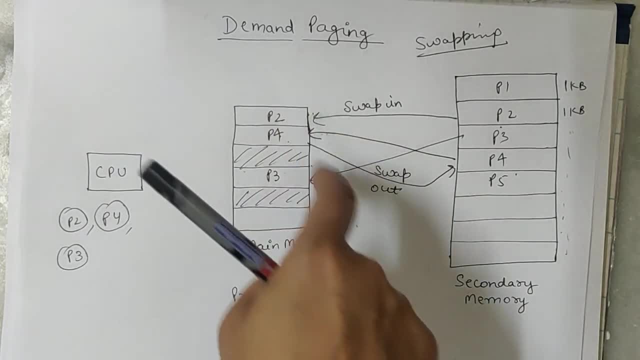 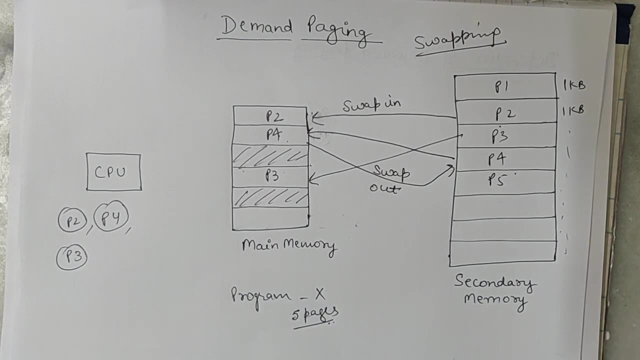 swap-out In demand paging is known as swapping. Suppose we have a program which finds out the cost of painting a room. In this program, when we have to find out the cost of painting a room, we have to find out the surface area of the room. 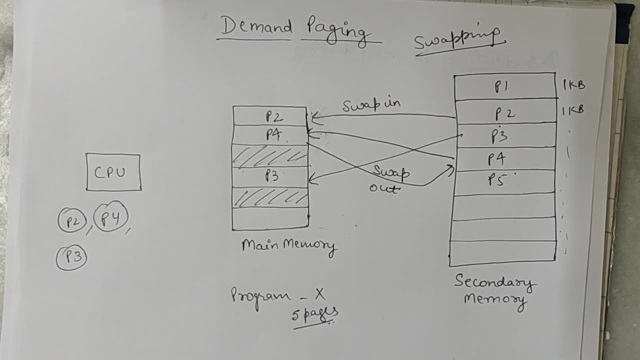 Suppose, the code to find out the surface area is in 6-10 instructions and the code to find out the surface area is in page 5 of the room And the formula to find out the cost is in page 1.. So the CPU will not find out the page 1 first.